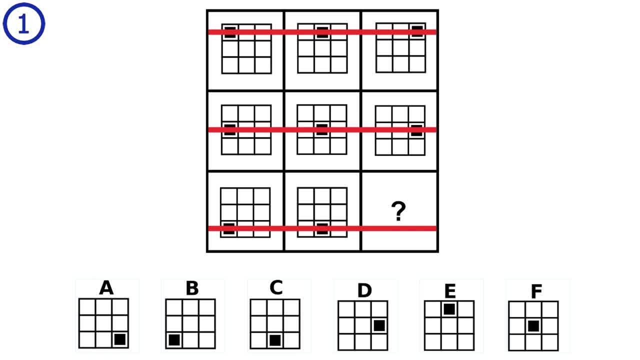 at the rows we can see that the black squares in the pictures are in the same rows as the pictures themselves are in. For example, in the first row we only have black squares in the first row in the pictures. in the second row we only have black squares in the second row in the pictures and in. 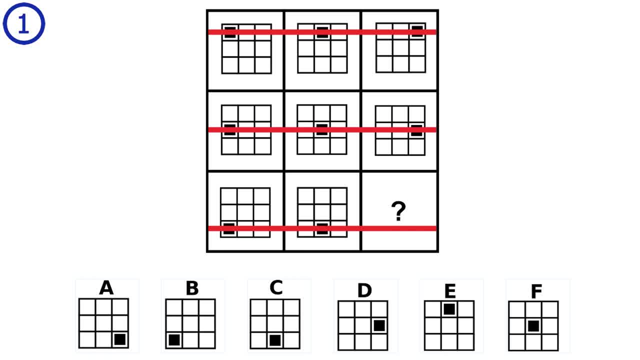 the third row. we only have black squares in the third row. Since the answer is in the third row, we know that our answer has a black square in the third row. Only answer A, B and C have their black square in the third row, so we can eliminate all the other answers. Now we can see the exact same. 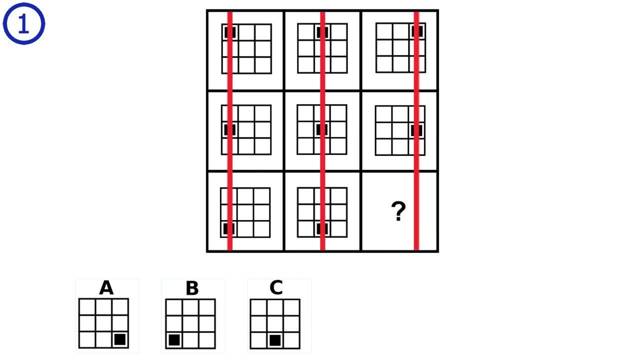 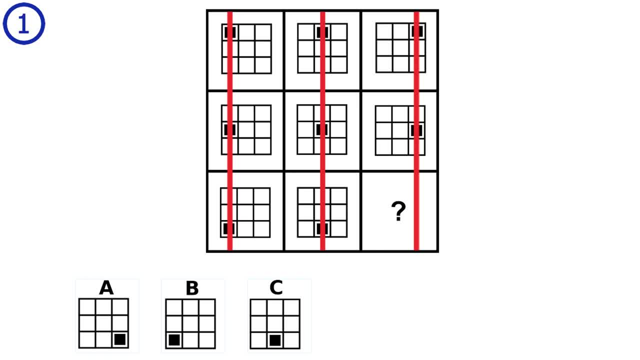 in the second column. we only have black squares in the second column and in the third column. we only have black squares in the third column. Since the answer is in the third column, we know that our answer will have a black square in the third column Out of the answers A, B and C. 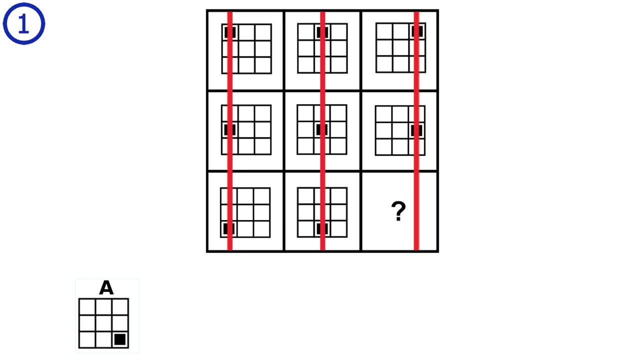 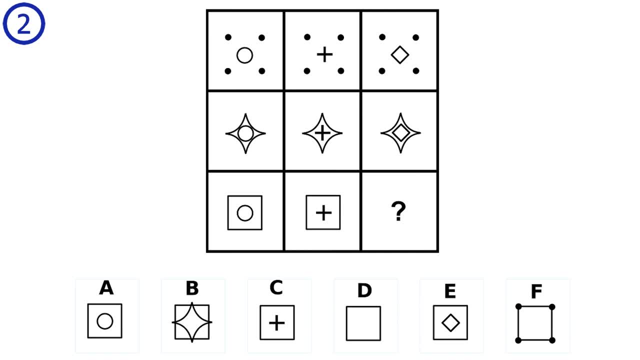 only answer A has a black square in the third column. Answer A is the correct solution. Puzzle number two: In this puzzle we have repetitions in the rows and the columns. In the first row we have a repetition of four black dots which are marked in red. 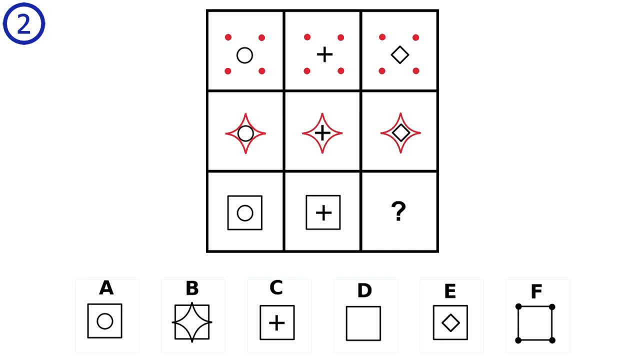 and in the second row we have a repetition of this star shape, and in the third row we have a repetition of squares. If we look at the answers, every single answer has a square, so we can't eliminate any answers yet. Now, if we look at the columns, we have a circle repeating in the first. 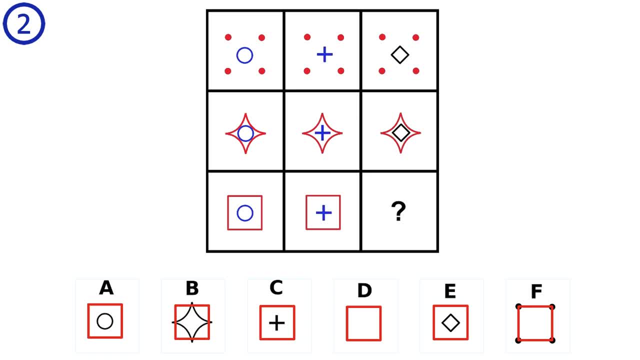 column which I'll mark in blue. In the second column there is a plus sign and in the third column we have this diamond shape. We know that our answer will have this diamond shape and if we look at the answers, only answer E has the diamond shape. Answer E is the correct solution. 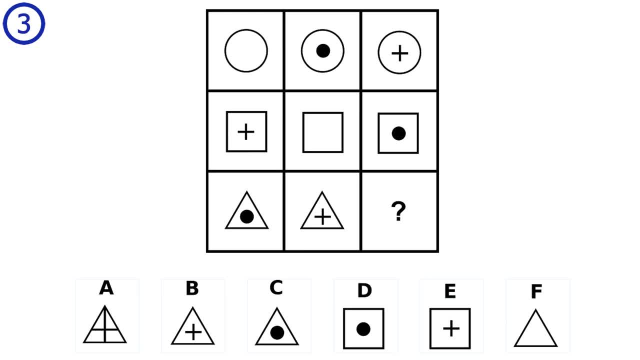 Puzzle number three. Starting off this puzzle, we see repetitions in the rows. In the first row we have circles, in the second row we have squares and in the third row we have triangles. Looking at the answers, only answer A, B, C and F has triangles, so we can eliminate the other answers. 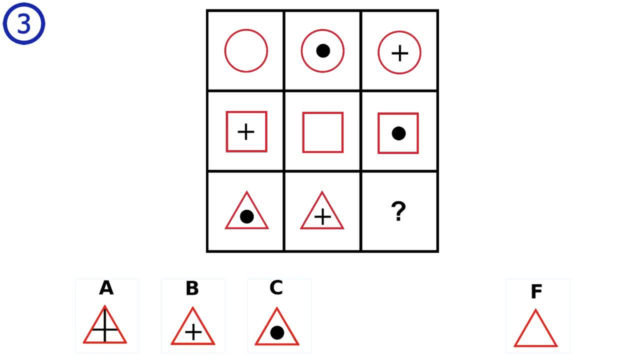 Now in this puzzle there aren't repetitions in the columns like in the previous puzzle. Here we have the repetitions in the diagonals from top left to bottom right. In the yellow diagonal we have a repetition of a plus sign. in the blue diagonal we have a repetition of this big dot and. 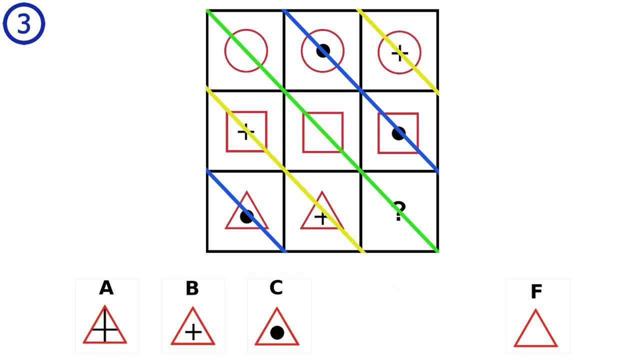 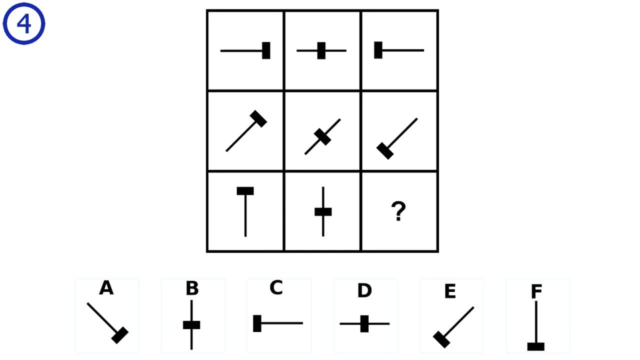 in the green diagonal, which the answer is in, we have a repetition of no inner shape. Looking at the answers, only answer F has no inner shape. Answer F is the correct solution. Puzzle number four: To solve this puzzle, I prefer to look at the columns. 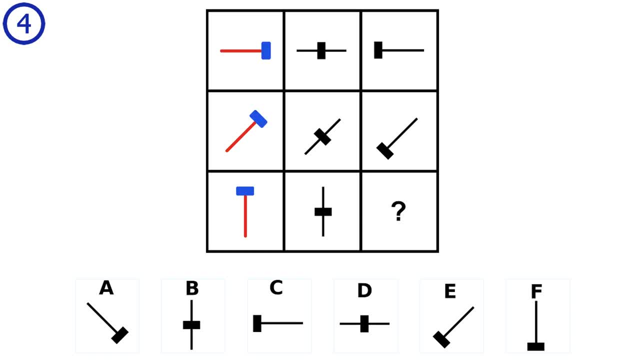 If we focus on the first column, we see that the shape is rotated by 45 degrees in counterclockwise direction as you move from picture 1 to picture 2 or from picture 2 to picture 3.. In the second column, we see the exact same rotation of 45 degrees in counterclockwise direction. 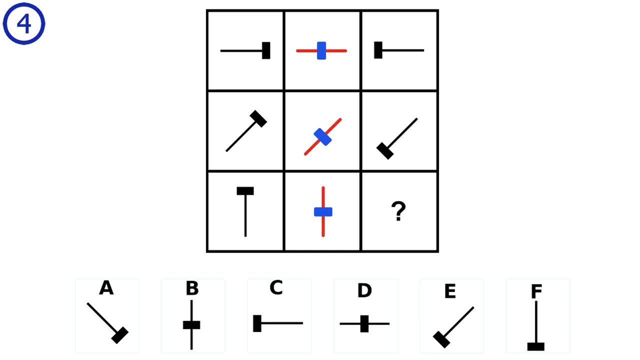 as we move that way down in the column. Therefore, we know that whenever we move downwards in a column, there is a rotation of 45 degrees in counterclockwise direction, independent of what column we look at. To solve the puzzle, we look at the second picture in the third column and we rotate. 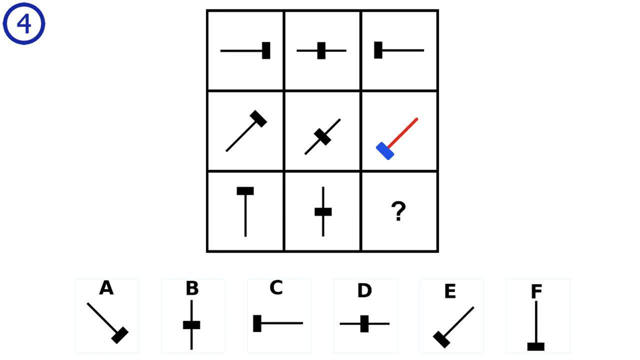 it by 45 degrees in counterclockwise direction. This will make a shape identical. to answer F. Answer F is the correct solution. Puzzle number 5.. This is pretty much exactly the same as the previous puzzle, but here we have a rotation. 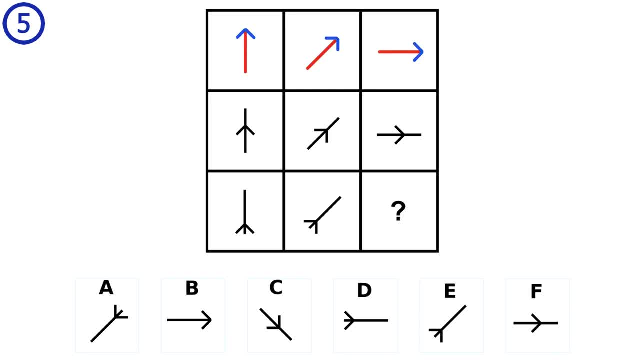 in the rows. Starting on the first row, we see that there is a 45 degree clockwise rotation going from picture 1 to picture 2, or from picture 2 to picture 3.. In the second row we have the exact same 45 degrees clockwise rotation as we move towards. 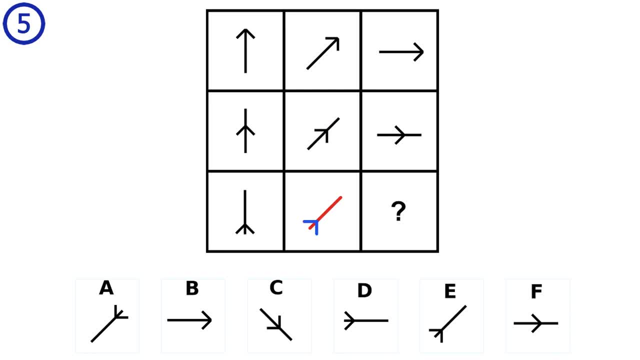 the right To solve the puzzle. we look at the second picture in the third row and we rotate it by 45 degrees in clockwise direction, which leads to a shape identical to answer D. Answer D is the correct solution. Puzzle number 6.. 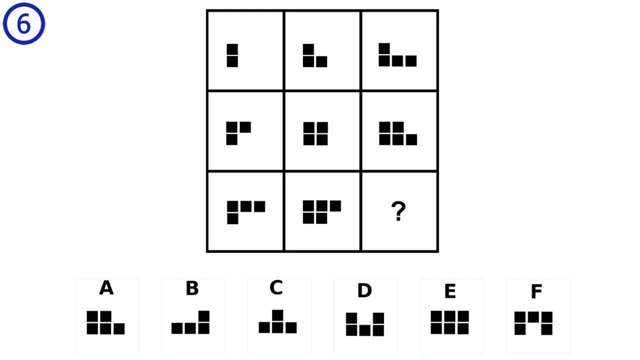 This is another puzzle where we have repetitions in the rows and the columns. Starting off, I want you to look at the row D: In the first row we have one square, in the second we have two and in the third we have 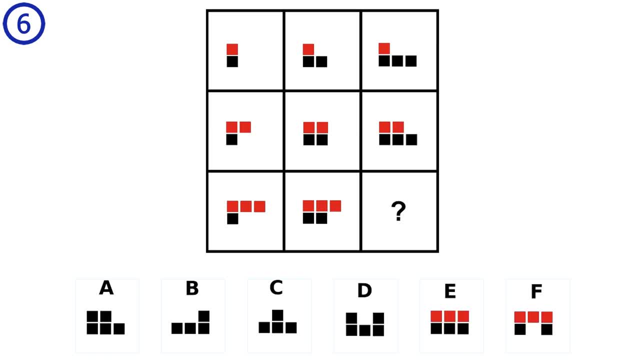 three. We know that our answer will have three squares in the top, so we can eliminate all the other answers. Next, I want you to focus on the columns and how many squares we have in the bottom of each picture. In the first column we have one, in the second we have two and in the third we have three. 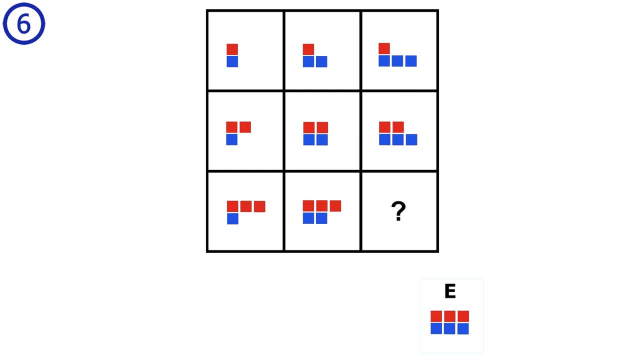 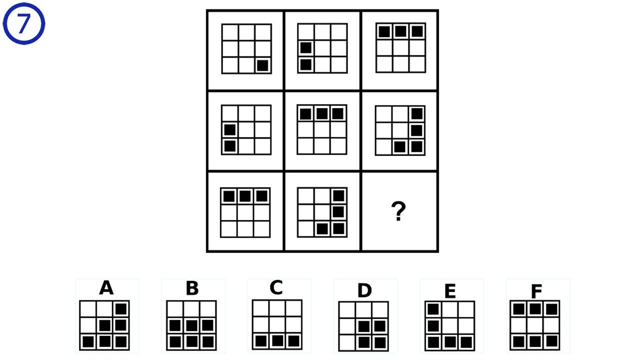 Answer E has three squares in the bottom. Answer E is the correct solution. Puzzle number 7.. In this puzzle we have the same effect. moving to the right In the first picture we have this square. If we rotate the entire picture by 90 degrees clockwise, we will get a square in the bottom. 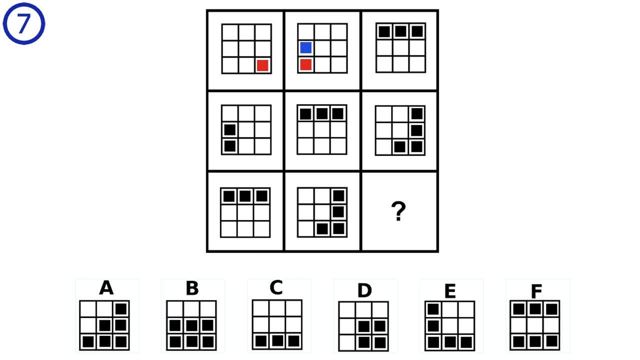 left corner, as we can see in picture 2.. We then add a new square in the first empty slot in the clockwise direction of the first square. The same thing happens when moving from the second to the third picture. We first rotate the entire picture by 90 degrees clockwise and then we add a new square in. 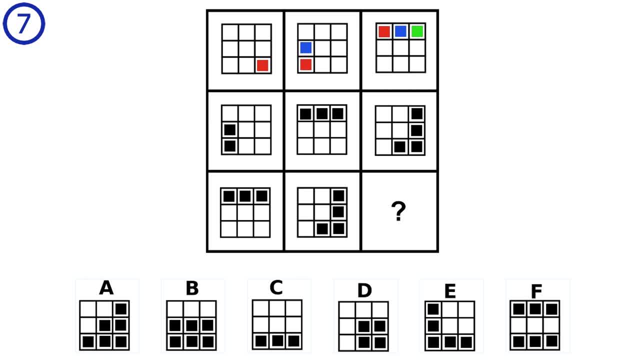 the first empty slot in the clockwise direction. To solve the puzzle. we do this for the second picture in the third row. Answer E is the correct solution. If we rotate the entire picture by 90 degrees clockwise, we get squares in the same positions. 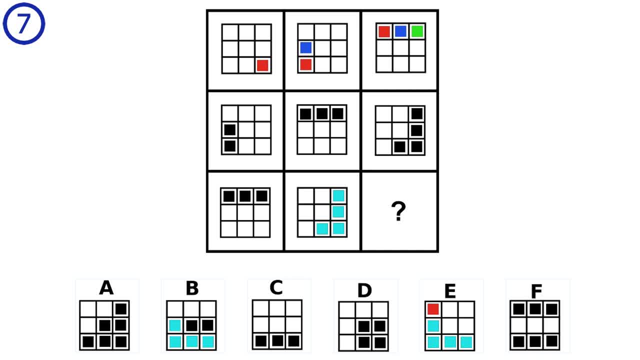 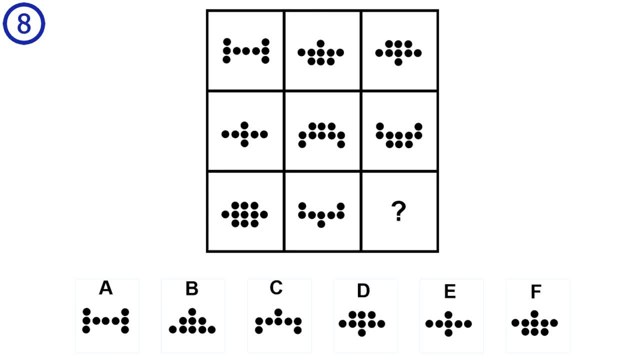 as we can see in answer B and answer E. Then we add a new square in clockwise direction, as we can see in answer E. Answer E is the correct solution. Puzzle number 8.. This is a puzzle with repetitions in both of the diagonals. 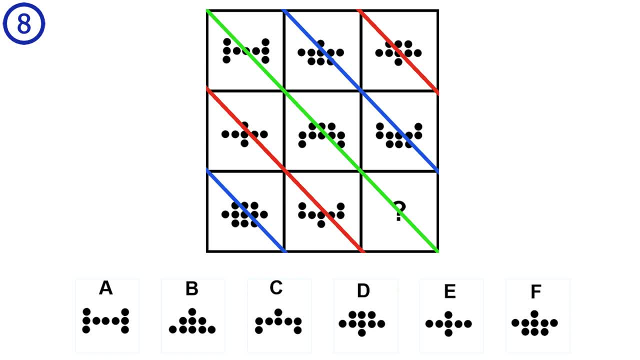 First, if we look at the diagonals from top left to bottom right, we can see a repetition of the bottom half of the pictures. Looking at the red diagonal, we see a repetition of a single dot in the middle bottom. In the blue diagonal there are three dots in the bottom. 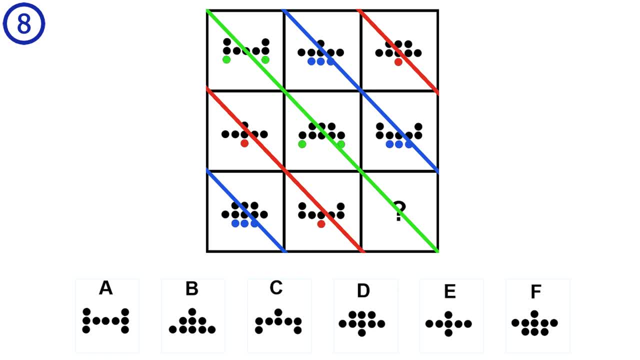 Which the answer is in. there are two dots on opposite sides of each other on the bottom. If we look at the answers, only answer A and C has the dots on opposite sides of each other on the bottom. So we can eliminate all the other answers. 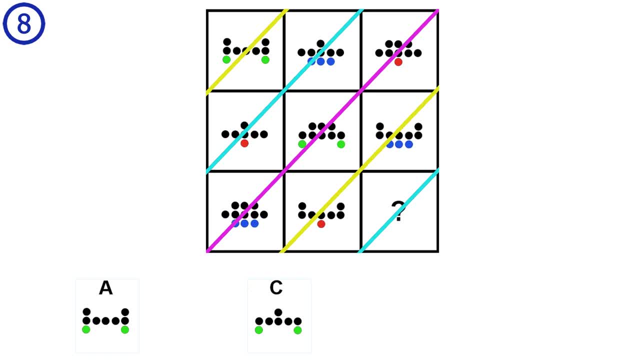 Next, if we look at the diagonals from top right to bottom left, there are repetitions in the top half of the pictures. In the yellow diagonal, we have two dots on the opposite sides of each other. In the purple diagonal, we have three dots in the middle. 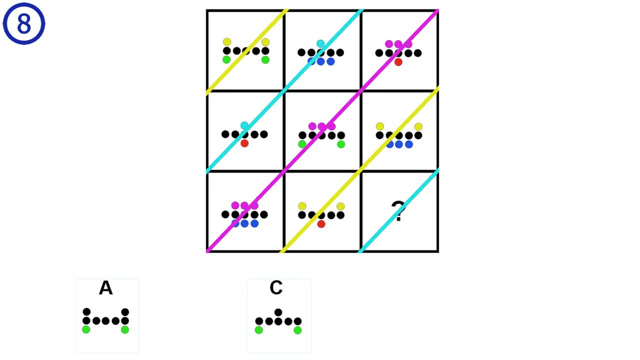 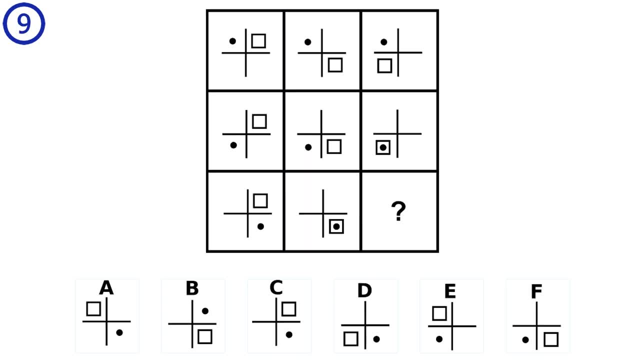 And in the light blue diagonal which the answer is in, we have a single dot in the middle. So only answer C has a single dot in the top half. Answer C is the correct solution. Puzzle number nine: This is a puzzle where we have repetitions in the rows and the columns. 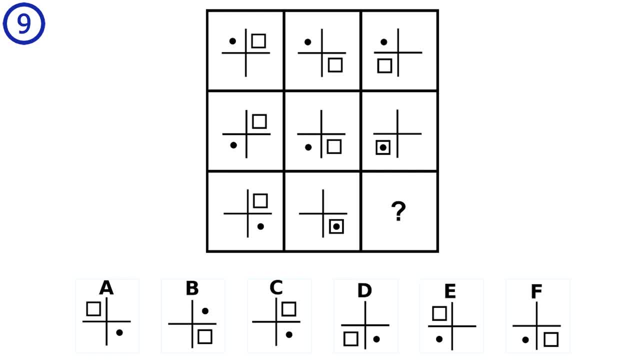 Starting off, we can see that there is a repetition of the black dot in the rows. In the first row the dot is in the top left, In the second row it's in the bottom left And in the third row it's in the bottom right. 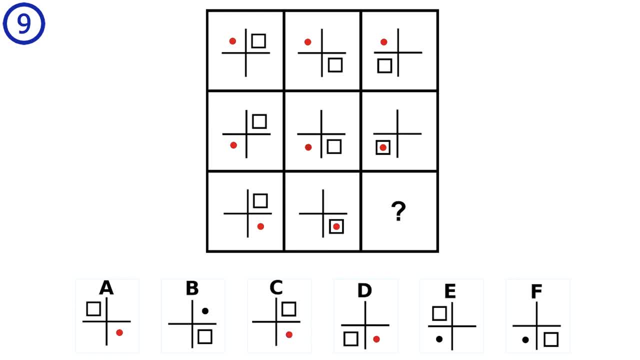 If we look at the answers, only answer A, C and D has a black dot in the bottom right So we can eliminate all the other answers In the columns. we have a repetition of the square In the first column. it's in the bottom right. 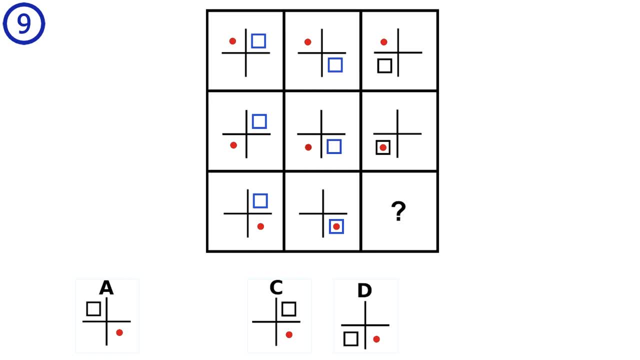 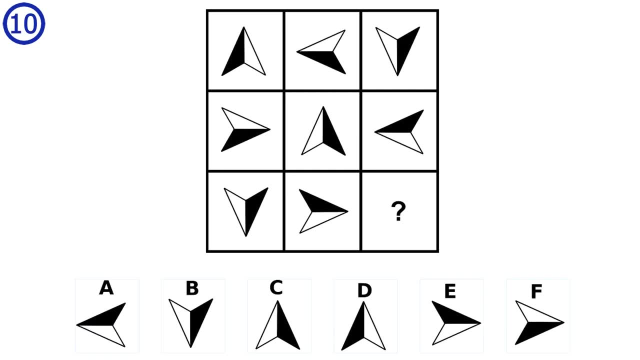 In the second column it's in the bottom right And in the third it's in the bottom left. Only answer D has a square in the bottom left. Answer D is the correct solution. Puzzle number ten. This is a rotation puzzle in the rows. 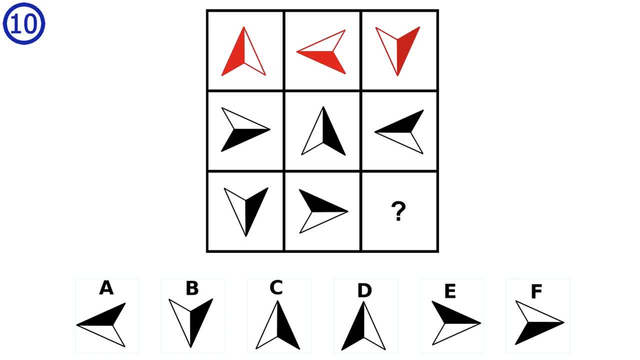 Looking at the first row, we have a 90 degrees counterclockwise rotation going from picture one to picture two and picture two to picture three. In the second row we have the exact same 90 degree counterclockwise rotation as we move. 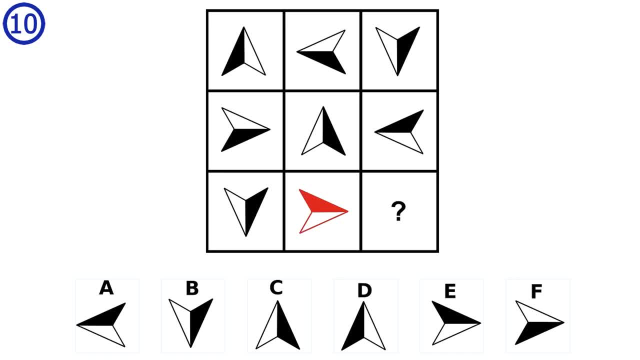 towards the right. To solve the puzzle, we look at the second picture in the third row and we rotate it by 90 degrees in counterclockwise rotation As in counterclockwise direction, which leads to answer D. Answer D is the correct solution. 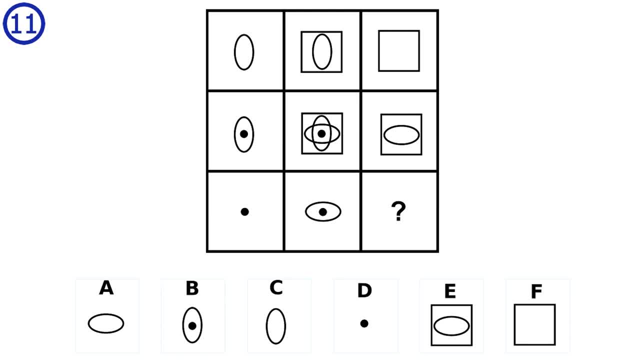 Puzzle number eleven. This is the first addition puzzle of the test. If we look at the first row, we have this vertical ellipse in the first picture, which we can also see in the second picture. In the third picture we have this square, which we can also see in the second picture. 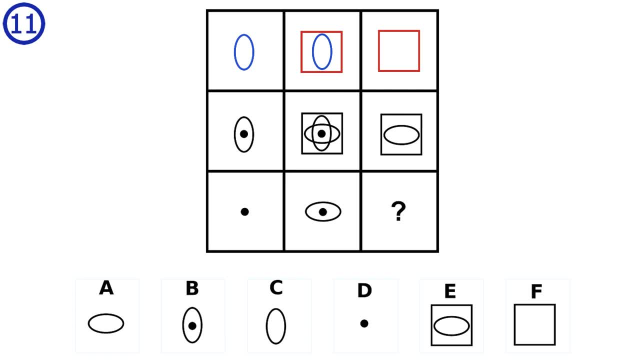 The second picture is simply the shapes in the first picture, added with the shapes in the third picture. In the second row we have these shapes in the first picture and these shapes in the third picture. We can see how adding them together leads to the second picture. 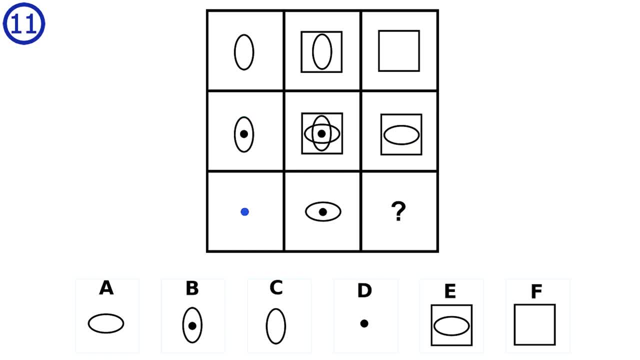 To solve the puzzle. we go by the third row In the first picture. we have this dot which we can also see in the second picture. Now the horizontal ellipse which you can see in the second picture is not in the first picture, so it has to be in the answer. 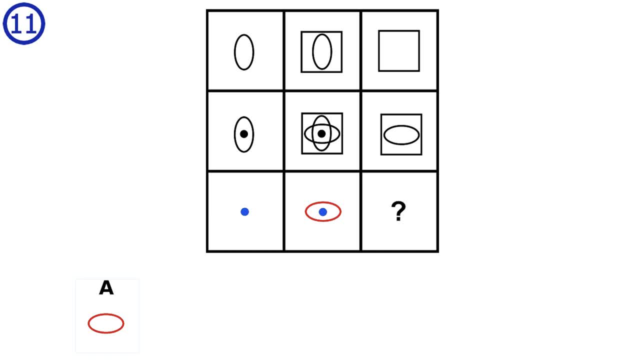 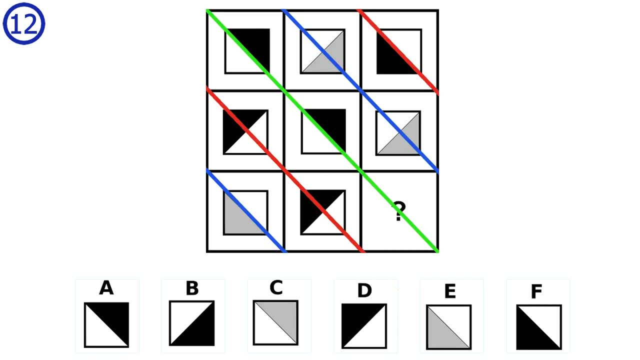 Answer A has a horizontal ellipse. answer A is the correct solution. Puzzle number 12.. Starting off this puzzle, we see that there is a repetition of color on the top left to bottom right diagonals. In the blue diagonal there are grey shapes, while in the red and green diagonal there. 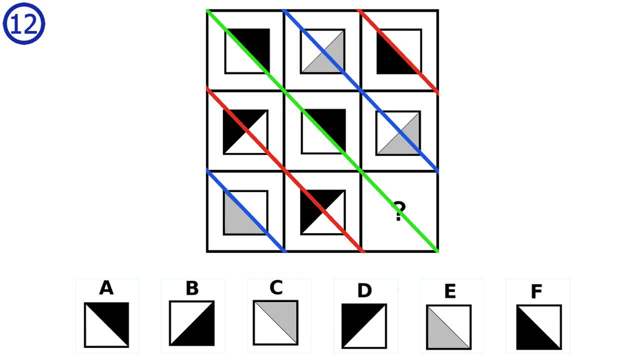 are black shapes. Our answer is in the green diagonal, so we know that the answer is a black shape. Therefore we can eliminate answer C and E. Because all the answers are the same color, we can ignore the color component of the puzzle. 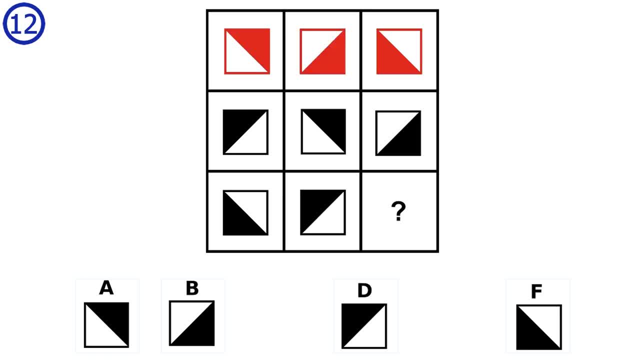 If we focus on the first row, we can see that there is a 90 degree clockwise rotation as we move towards the right in the row. In the second row we have the same 90 degree clockwise rotation as we move towards the right. So to solve the puzzle, we go by the second picture in the third row and rotate it by. 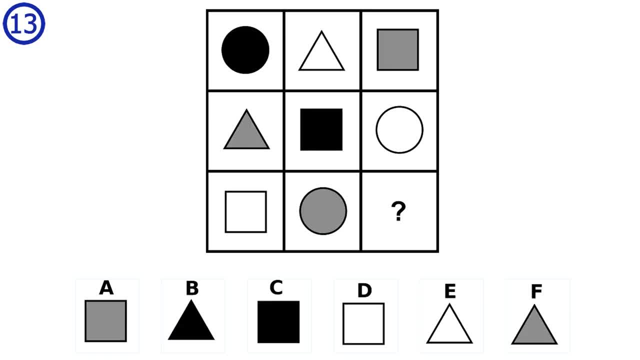 an increased degree. clockwise. Answer A is the correct solution. Puzzle number 13.. Starting off, we look at the top left to bottom right diagonals and we see that there is a repetition of dark black color on each of the diagonals. In the green diagonal, where the answer is in, there is a repetition of black shapes. 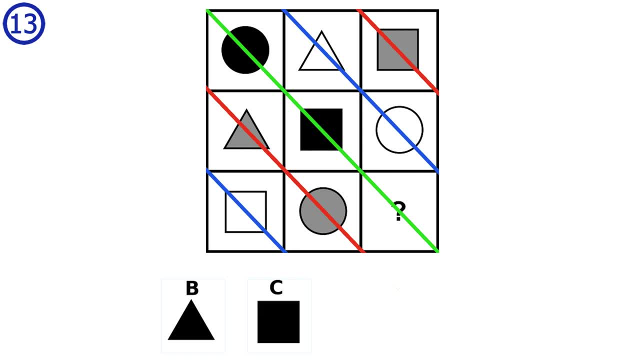 We can eliminate every non-black shape answers, leaving answer B or C as correct. Next, let's look at the bottom right to bottom right diagonal. In these diagonals there is a repetition of the shapes themselves. In the light blue diagonal, which the answer is in, there is a repetition of darker skinned. 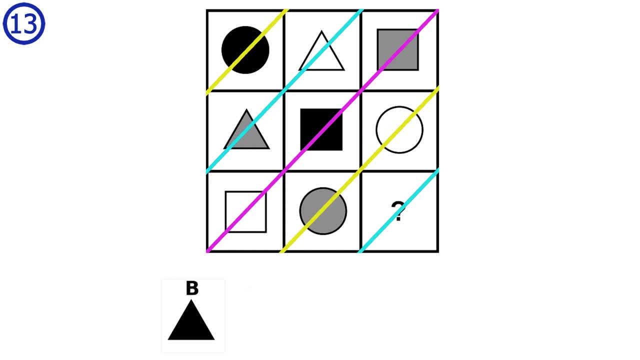 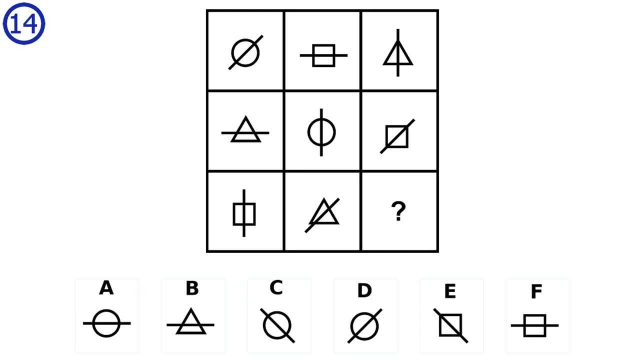 shapes of triangles. so the answer is a triangle. Answer b is the correct solution. Puzzle number 14.. This puzzle is exactly the same as the previous puzzle, with repetition in both of the diagonals, In the top left to bottom right diagonals, we have a repetition. 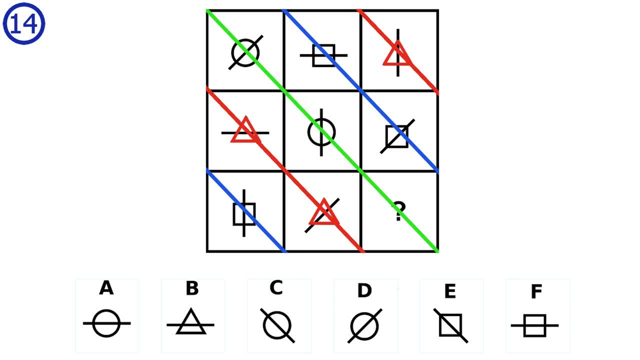 of the main shapes. In the red diagonal there are triangles, in the blue diagonal there are squares and in the green diagonal, which the answer is in, there are circles. Only answer a, c and d have circles, so we can eliminate all the other answers. Next, if we look at: 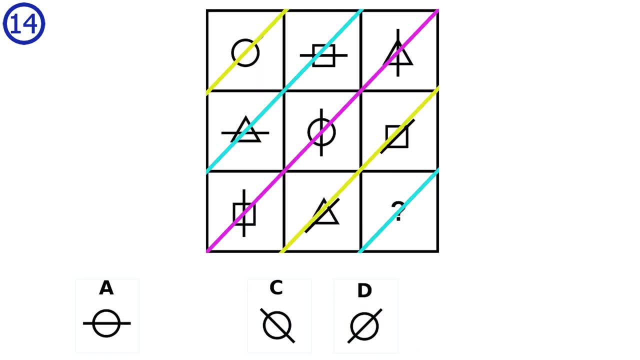 the top right to bottom left diagonals we have a repetition of the lines. In the light blue diagonal, where the answer is in, we have a repetition of a horizontal line. Out of the three answers, only answer a has this horizontal line. Answer a is correct. 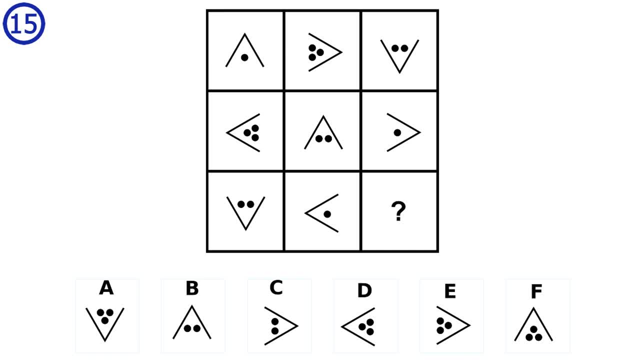 Puzzle number 15.. The black dots in this puzzle repeat in the diagonals from top right to bottom left. In the yellow diagonal there is one dot per picture, in the purple diagonal there is two and in the light blue there is three. The answer is in the light blue diagonal. 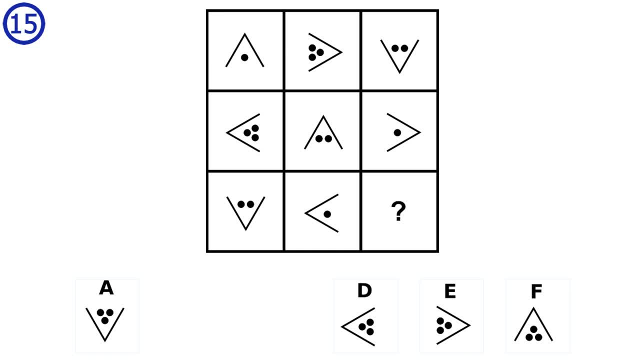 so we know that the answer will have three dots. To simplify the puzzle, we can use the following rules: We can just remove every dot, since every answer has the same amount of dots. Now, it's just a simple rotation puzzle. In the first row we can see a 90 degrees clockwise rotation. 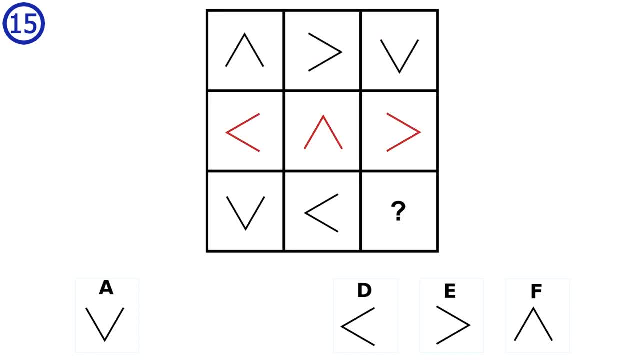 as we move towards the right In the second row we see the same 90 degree clockwise rotation. so to solve the puzzle we just rotate the second picture in the third row by 90 degrees clockwise. This leads to the arrow pointing upwards. Answer f is the correct solution. 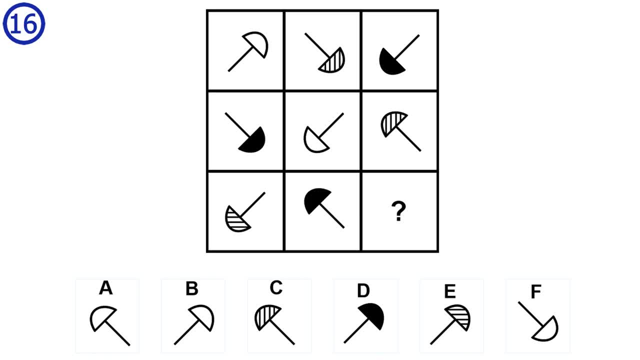 Puzzle 16.. This puzzle is very similar to the previous puzzle. If we look at the diagonals from top left to bottom right, We can see that the pattern inside of the half circle in the pictures repeat on these diagonals. In the green diagonal where the answer is, there is a repetition of white half. 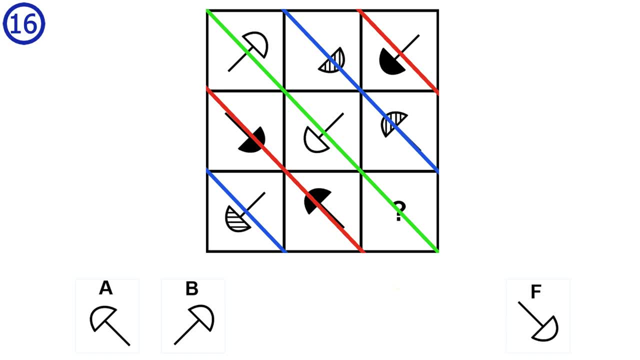 circles. This leaves only answer a, b and f as possible correct answers. Again, to simplify the puzzle, we can just remove the color component of the puzzle. Looking at the first row, we see that there is a 90 degree clockwise rotation as we move towards. 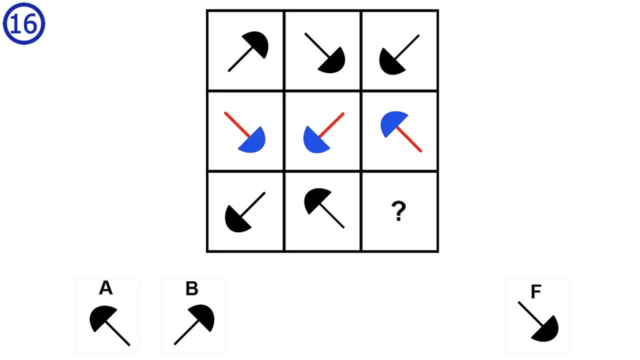 the right and we can see the same rotation in the second row. To solve the puzzle, we just rotate the second picture in the third row by 90 degrees clockwise, which gives answer b. Answer b is the correct solution: Puzzle 17.. This is a rotation puzzle. I prefer looking at the columns in this puzzle In. 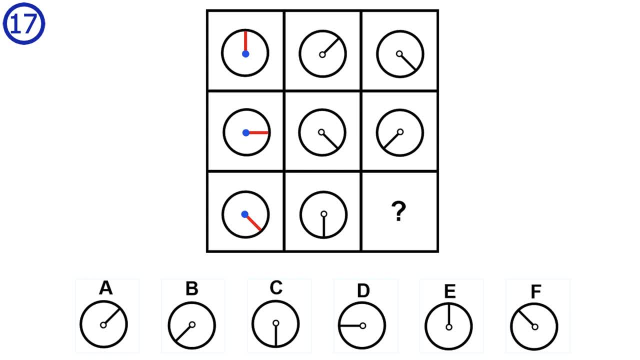 the first column we first have a 90 degree clockwise rotation going from picture 1 to picture 2, and then we have a 45 degree clockwise rotation going from picture 2 to picture 3.. In the second column we have the exact same thing: First 90 degrees, then 45 degrees. both 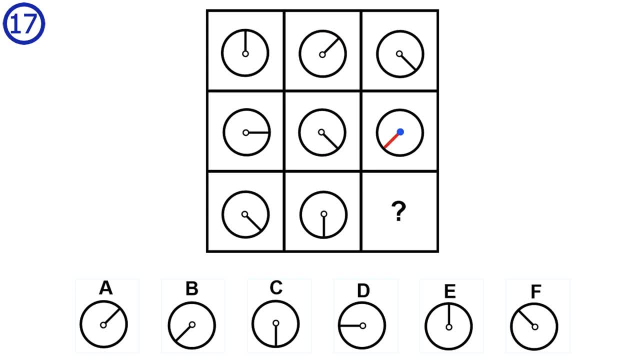 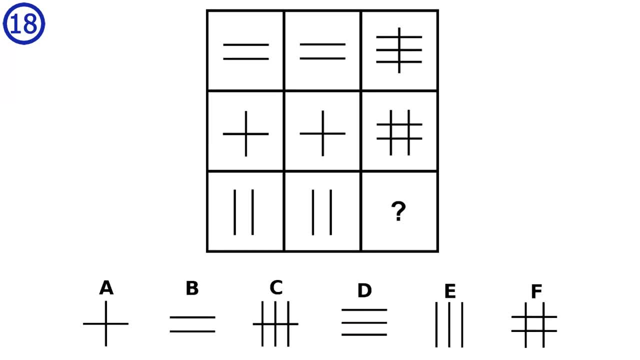 in clockwise direction. To solve the puzzle we go by the second picture in the third column and rotate it by 45 degrees in clockwise direction. Answer d is the correct solution. Puzzle number 18.. In this puzzle we just have to count the amount of horizontal and vertical. 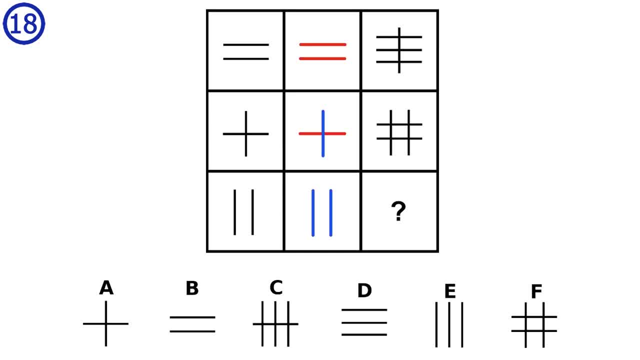 lines. If we look at the second column, we see that as we move downwards in the column, the horizontal lines are converted into vertical lines. First we have 2 horizontal and 0 vertical, then we have 1 horizontal and 1 vertical and finally 0 horizontal and 2 vertical. Looking 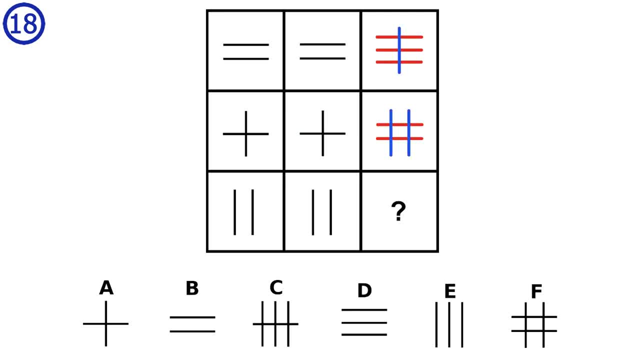 at the third column we see the exact same effect of transforming horizontal lines into vertical lines, one at a time. In the second picture we have 2 horizontal and 2 vertical lines, so the answer should have 1 horizontal line and 3 vertical lines. Answer c is the correct solution. 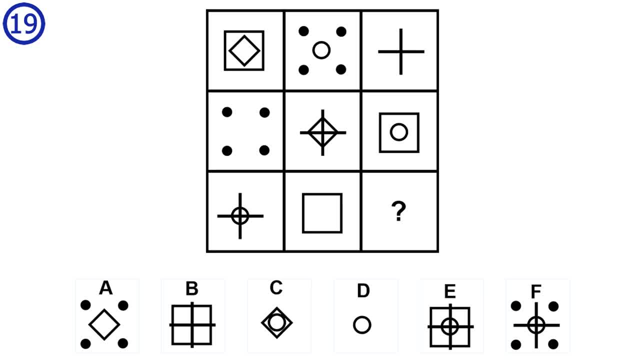 Puzzle number 19.. In this puzzle we see the repetition in both of the diagonals: In the top left to bottom right diagonals. we see the repetition of shapes. In the green diagonal, which the answer is in, we see the repetition of this diamond shape which you can see in. 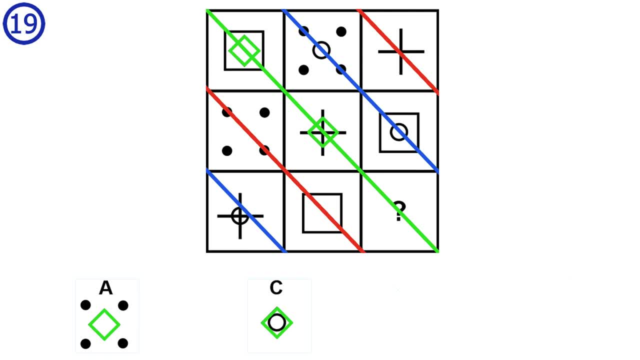 answer a and c. We can just remove the rest of the answers. In the top right to bottom left diagonals there is also a repetition of shapes. In the bottom left to bottom right diagonal which the answer is. in there is a repetition of these 4 dots. The same 4 dots can be seen in answer a. Answer a is the correct solution. 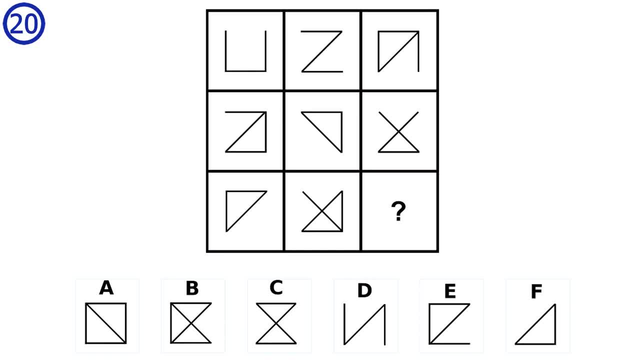 Puzzle number 20.. The way it works is that we take the lines which is not in common between the two first pictures in a row or column and we add them together to create the third picture. For example, if we look at the first row, the two first pictures have these lines: 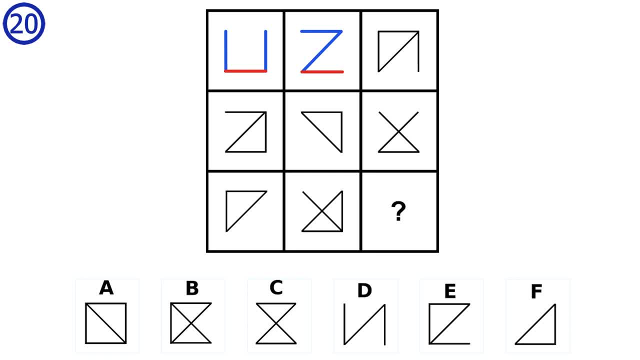 not in common and this line in common. To create the third picture, we just take the blue lines from the first picture and add them with the blue lines from the second picture. To confirm this pattern we have to look at the second row. The two first pictures have 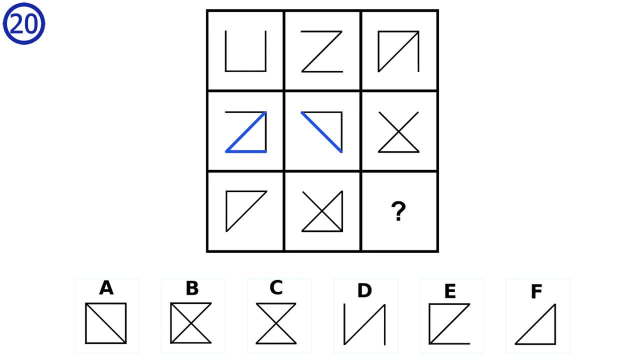 these lines not in common and adding them together gives picture 3.. To solve the puzzle, we follow this pattern for the third row. The two first pictures have these lines not in common and adding them together gives a picture identical. to answer a Answer: a is. 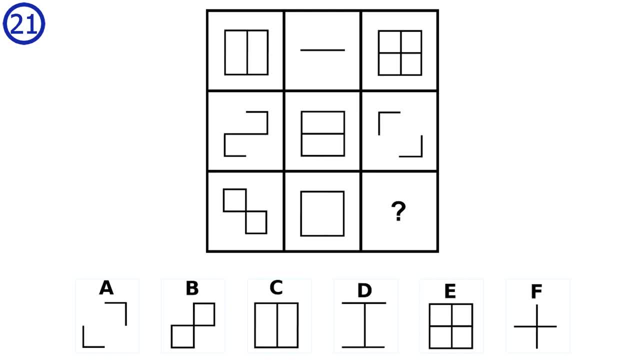 the correct solution. Puzzle number 21.. This is the exact same puzzle as the previous one. If we look at the first row, the two first pictures have these lines not in common and adding them together gives picture 3.. For the second row, we have these lines not in common and this line in common. 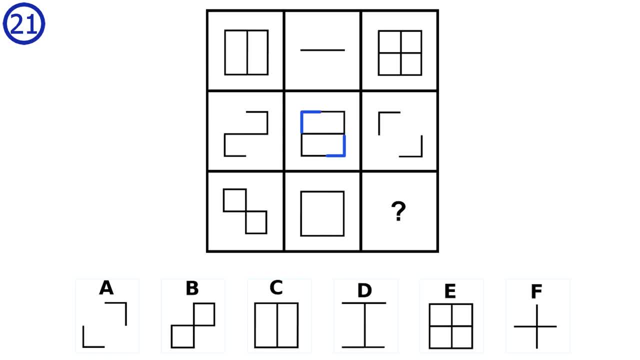 To solve the puzzle. we follow this pattern. for the third row. The two first pictures have these lines not in common and they produce picture 3.. For the third row: we have these lines not in common and adding them together gives answer b. Answer b is the correct solution. 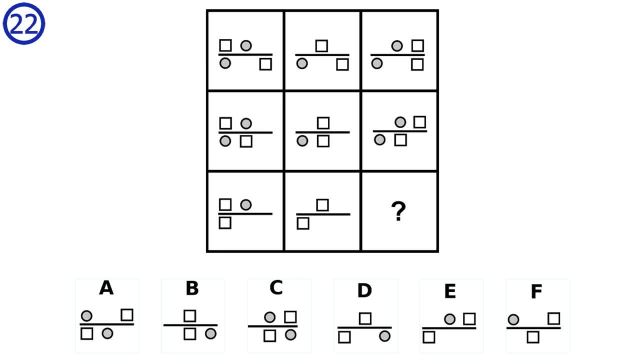 Puzzle number 22.. This is a repetition puzzle where we have repetitions in the rows and the columns. If we look at the rows and the lower half of the pictures, we see that in the first row we have a circle on the left and a square in the right. In the second row, 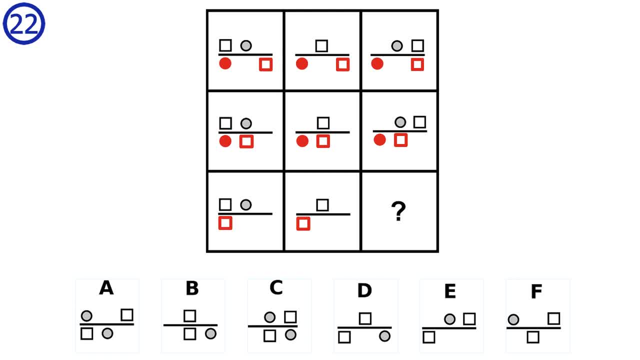 we have a circle on the left and a square in the middle, And in the third row we have a square on the left. Out of all the answers, only answer e has a square on the bottom left. Answer e is the correct solution. Before moving to the next puzzle, I would just like to point out that 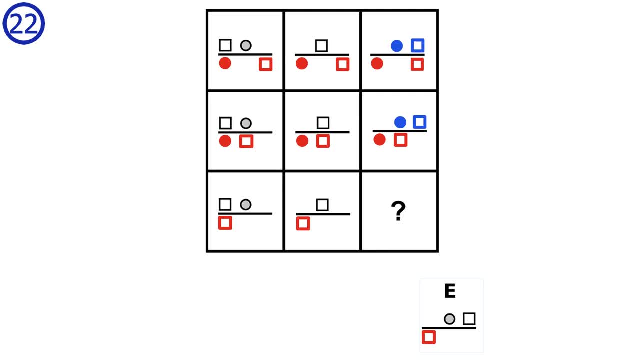 the top half repeats in the columns and if we look at the third column we have a circle in the middle and a square on the right, which we can also see in answer e Puzzle number 23.. In this puzzle I see repetitions on the top right to bottom left diagonals. 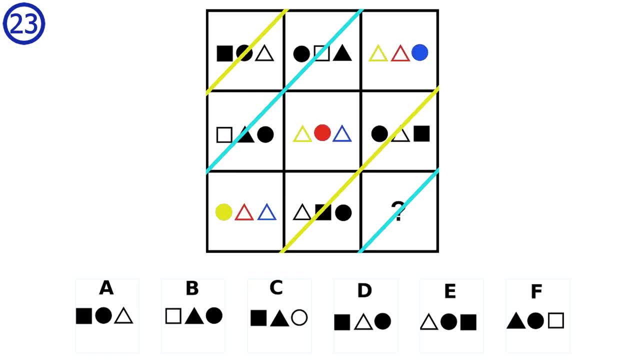 If we look at the purple diagonal and look at the position of each of the shapes, we see that as we move down in the diagonal, the circle moves to the left. To solve the puzzle, we we look at the light blue diagonal. we can see that moving from picture 1 to picture 2, the triangle- 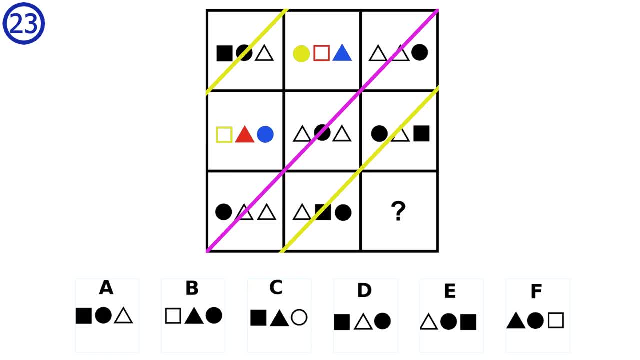 moves left to the middle position, the square moves left to the left position and the circle moves left and reappears on the rightmost position. To solve the puzzle, we have to base ourselves on the second picture in the diagonal and move the shapes once towards the left. The circle moves. 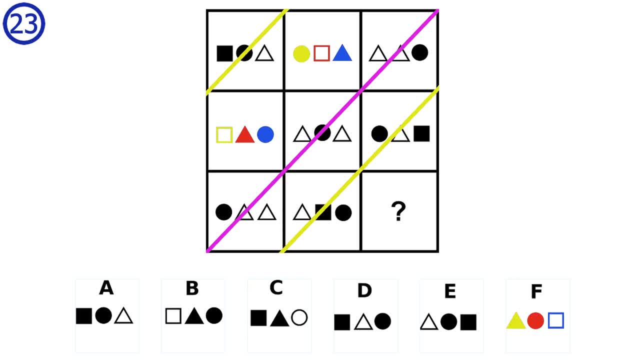 left to the middle position, the triangle moves left to the left position and the square moves left and reappears in the right position. Answer F is the correct solution. Puzzle 24.. This is an addition puzzle of the lines which the two first pictures do not have in common In the first row. 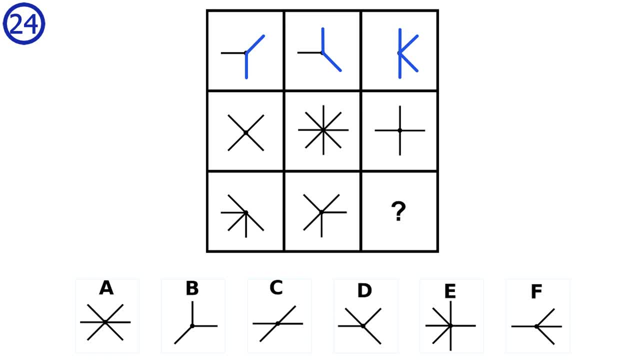 we have these lines not in common and added together produces picture 3.. In the second row we have these lines and they produce this picture, and in the third row we have these lines not in common between the two first pictures and adding them together gives answer F. Answer F is the. 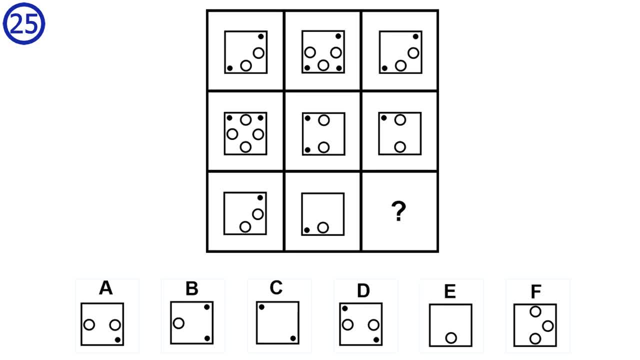 correct solution: Puzzle 25.. In this puzzle we look at what the two first pictures have in common rather than what they do not have in common. For example, in the first row we have these two shapes not in common And these shapes in common. We can see that picture 3 is simply the shapes which they have. 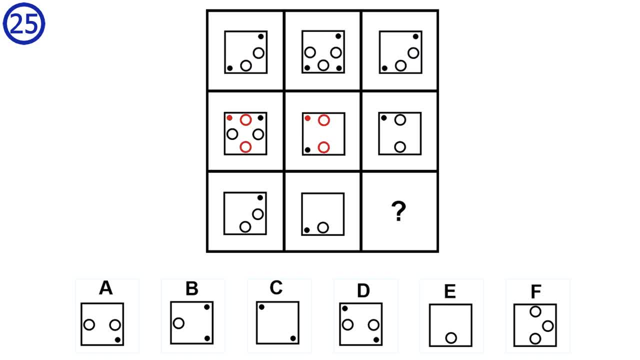 in common. In the second row we have these shapes in common, which is identical to the third picture. To solve the puzzle, we look at the third row and we see that all the two first pictures have in common is this circle on the bottom. If we look at the answers, only answer E has this circle on. 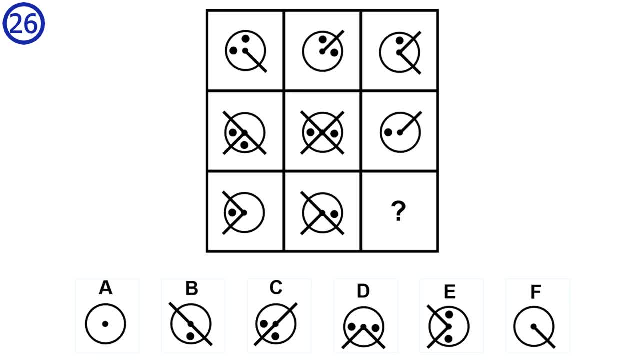 the bottom. Answer E is the correct solution. Puzzle 26.. For the dots in this puzzle, what is in common between the two first pictures is in the third picture, but for the lines, what is not in common between the two first pictures is in the third picture. For example, if we look at the first, 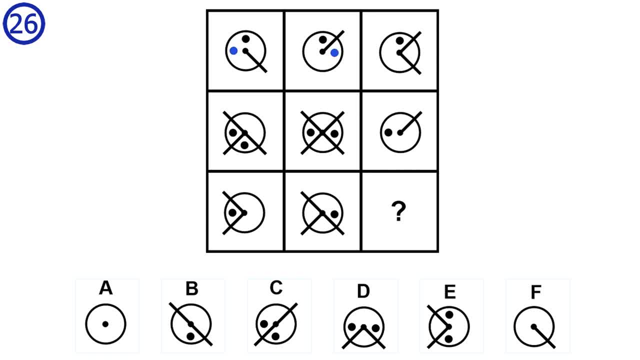 row and the two first pictures. we have these two dots not in common and these two in common. The dot in common is put into the third picture For the lines. we have these two lines not in common and they're both added to the third picture For the second row. we have this dot in common which 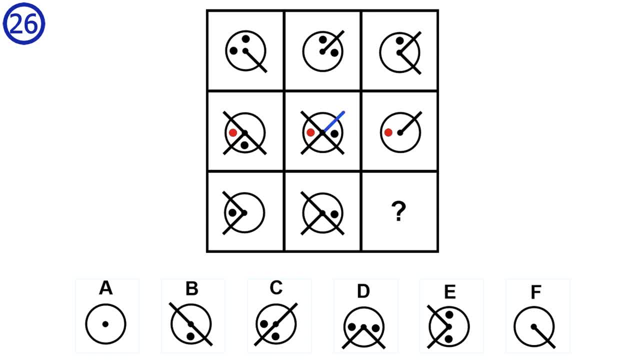 you can see in the third picture and for the lines we have this line not in common which you can see in the third picture. To solve the puzzle, we do this for the third row, The two first pictures. the answer will not have a dot For the lines we have this line not in common, which matches answer. 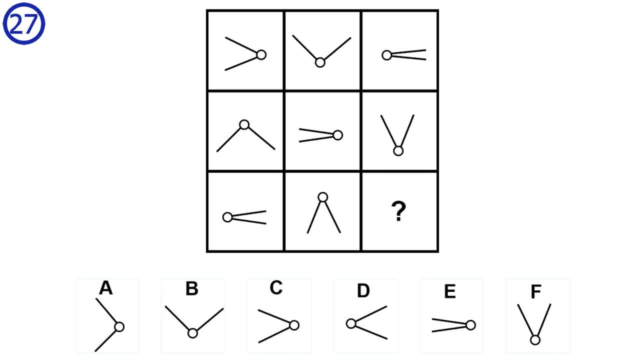 F. Answer F is the correct solution. Puzzle number 27.. In this puzzle I want you to pay attention to how wide the angle is between the two lines in each picture. To make it easier to see, I color coded the different angles: The least wide are red, the middle wide are green and the most wide 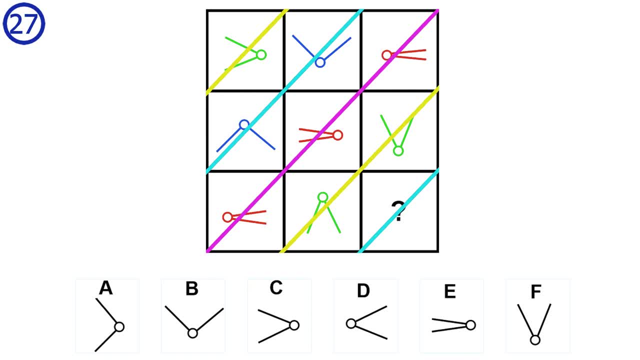 are blue. This is a repetition in the top right to bottom left diagonals and in the light blue diagonal we have the widest opening. Looking at the answers, only answer a and b have the widest opening, so we can eliminate the rest of the answers. Next I want: 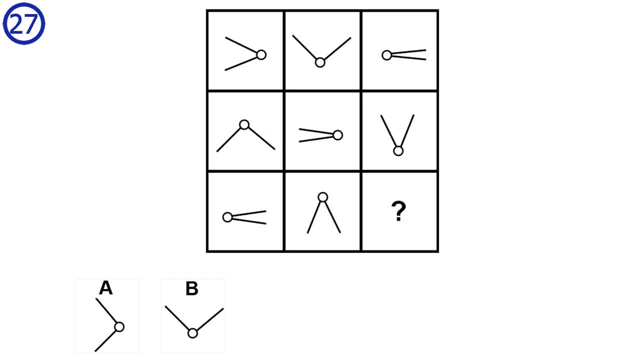 you to pay attention to what direction the opening in each picture are pointing towards. If we look at the first row, we can see that the directions of the pictures are rotated by 19 degrees in clockwise direction as you move towards the right. In the second row, we have the exact same 90 degrees. 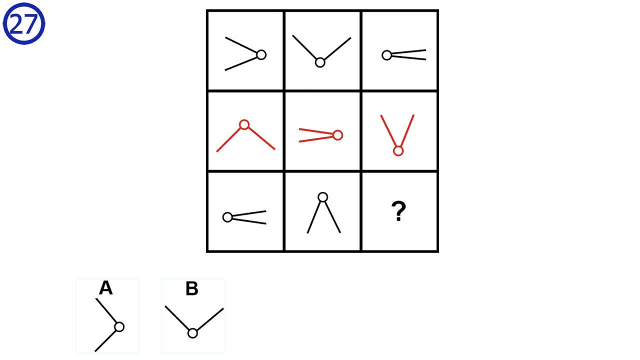 clockwise rotation as you move towards the right. To solve the puzzle, we have to look at the second picture in the third row and rotate it by 90 degrees in clockwise direction, which leads to the opening pointing towards the left. Before we move on with the puzzle, we have to look at the three 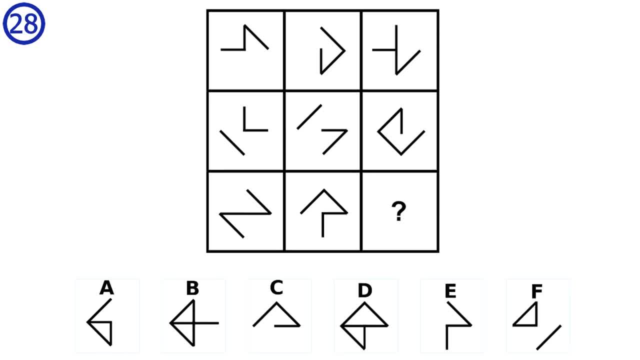 left. Answer A is the correct solution. Puzzle 28.. This is an addition puzzle where we add together what is not in common between the two first pictures to produce the third picture. In the first row we have these lines not in common and adding them together leads to picture 3.. In the 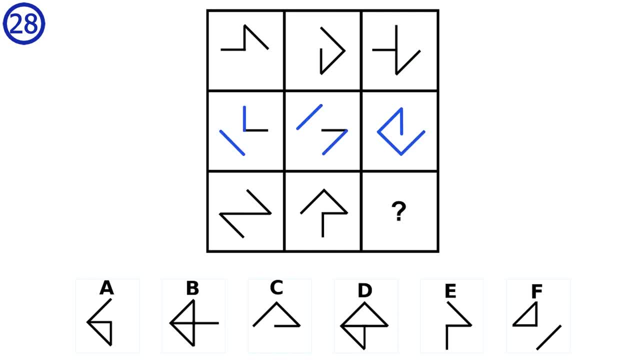 second row. we have these lines not in common and adding them together leads to picture 3.. To solve the puzzle, we do the same for the third row. We have these lines not in common and adding them together gives answer A. Answer A is the correct solution: Puzzle 29.. This puzzle is similar to an. 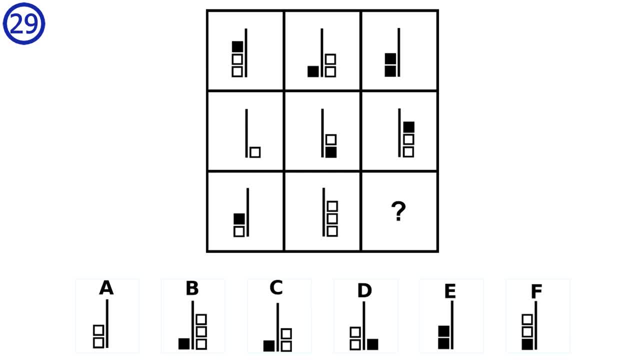 addition puzzle. Each picture has a line and two sides of the line. We add together the two first pictures in the row or column and if there is a similar shape on different side of the lines, the similar shapes cancel out. For example, if we look at the first row, the first picture have two. 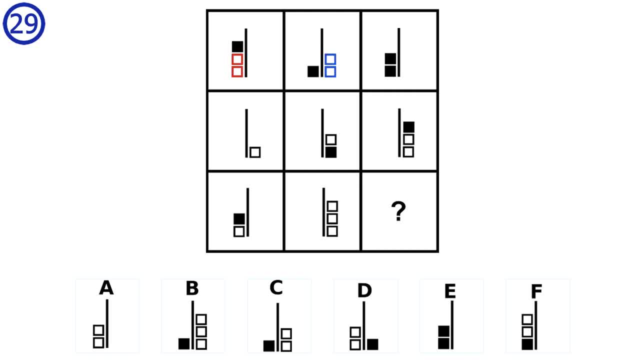 squares on the left side and the second picture has two squares on the right side. When we add together the two first pictures, the squares will cancel out and we will have no squares at all in the second row. If we add together the two first pictures, the squares will cancel out and we will 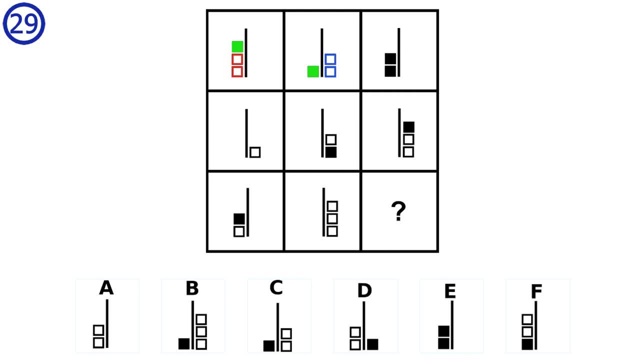 have no squares at all in the second row For the boxes. we have two boxes on the left side of the line and adding them together gives two boxes on the left side in the third picture. To solve the puzzle, we go by the third row. We have one square on the left side and three squares on the right. 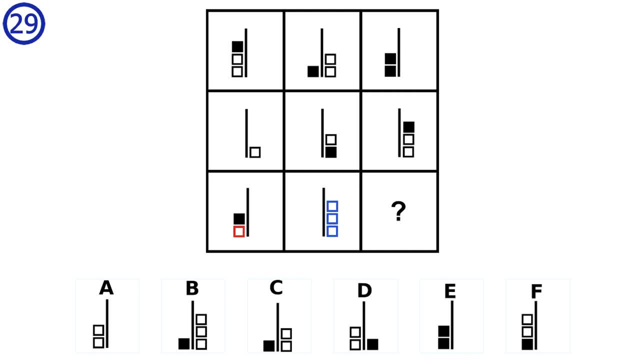 side. This means that one square will cancel out and we will be left with two squares on the right side in the correct answer. Only answer C has two squares on the right side. Answer C is the correct solution. Before going to the next puzzle, we can also see this box on the left side in the 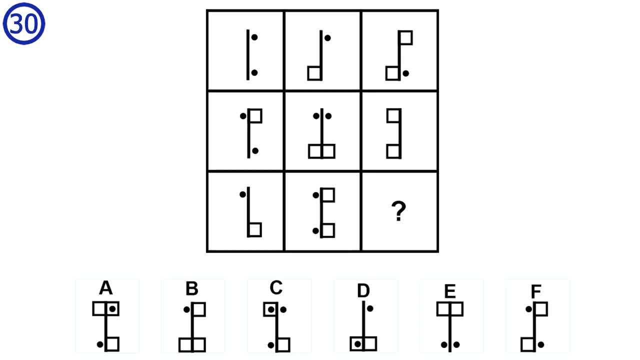 first picture, which you can also see on the left side in answer C Puzzle number 30.. This is another kind of addition puzzle. We have four positions and three objects which can be in the position. We have a black dot, a square or nothing at all. In order. 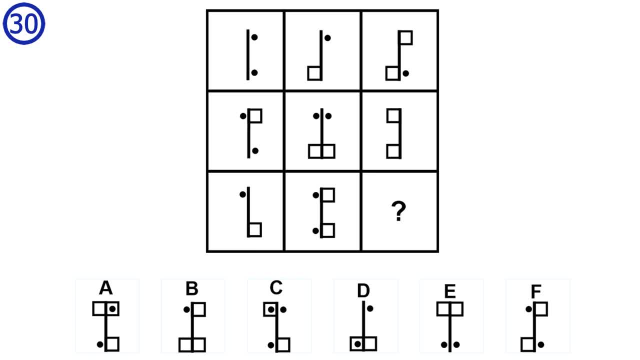 to solve the puzzle we have to figure out all the addition rules of the different objects. In the first row we can see that there are two dots in the top right in picture one and picture two, followed by a square in picture three. So we know that dot plus dot equals square. Again, using the 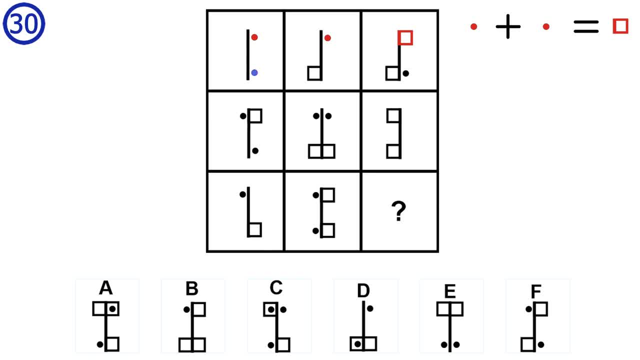 first row, we can see that on the bottom right we have a dot, nothing at all and a dot. So we know that dot plus nothing equals dot. Again, using the first row, in the bottom left, we have nothing, square, square. So we know that square plus nothing equals square. The two last: 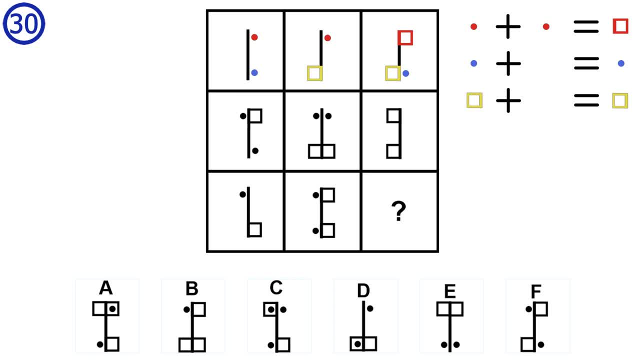 rules can't be found in the first row. The first of the two rules can be found in the second row, in the top right. We have a square, a dot and nothing at all. So we know that square plus dot equals nothing. The last rule can't be found in the rows. 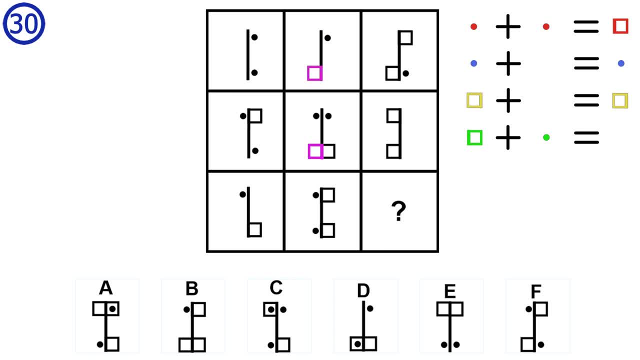 Instead, we have to look at the second column In the bottom left. we have a square, a square and a dot. So the final rule is that a square plus a square equals a dot. To solve the puzzle, we have to use these rules in the third row or third column. I prefer using 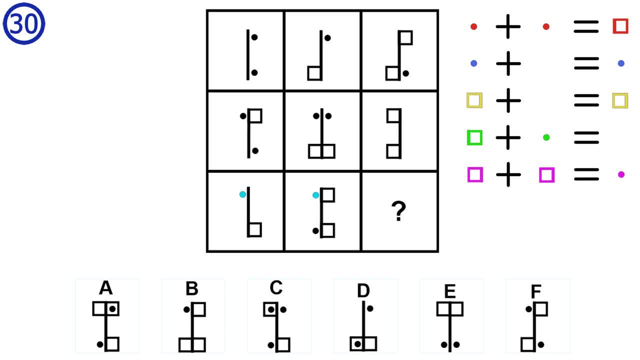 the third row, In the top left, we have a dot plus a dot equaling a square. Out of the six answers, only answer A and E has a square in the top left. In the bottom left we have a dot plus nothing equaling a dot, which you can see in both the answers. In the bottom right we have a square plus. 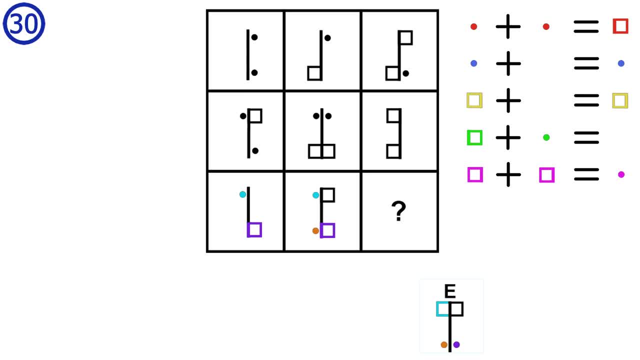 a square equaling a dot, which we can only see in answer E. Answer E is the correct solution For the top right. we would have a square plus nothing equaling a square, which you can also see in answer E. Puzzle 31: This is actually the replacement puzzle of the old puzzle 31 of the IQ test. The creator. 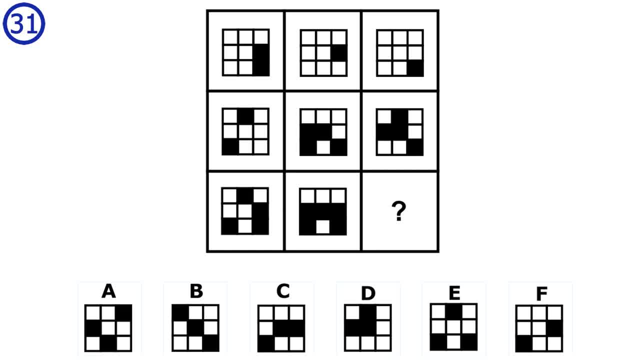 of the IQ test contacted me after watching a couple of my videos and I asked him if there was an official way to solve the old puzzle 31.. After he explained how to solve it to me, I pointed out a mistake in the puzzle and he replaced the old puzzle 31 with this. 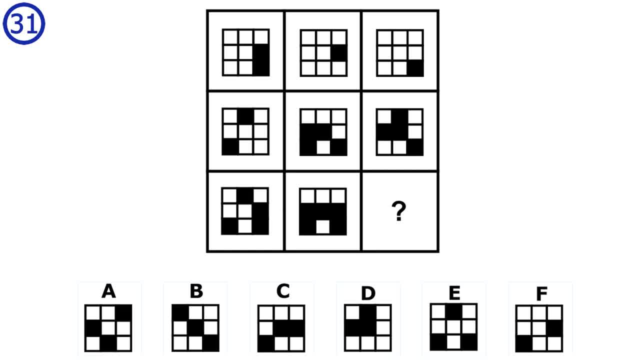 puzzle. My next video will be about the old puzzle 31,. what was wrong with the puzzle and how people attempted to solve an impossible puzzle. For the new puzzle 31, we have a simple addition puzzle. In the first row we have this square. 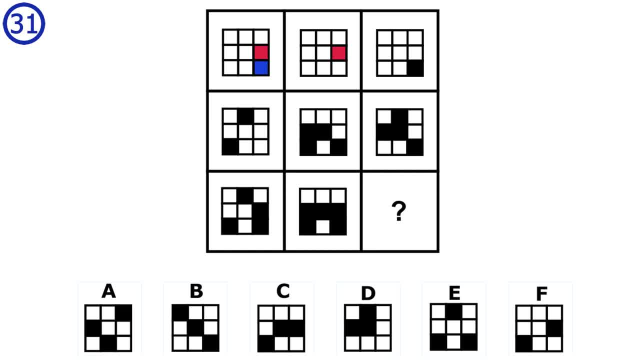 in common and this square not in common. This square, which is not in common, can be seen in the third picture For the second row. the two first pictures have these squares not in common and adding them together produces the third picture. To solve the puzzle, we 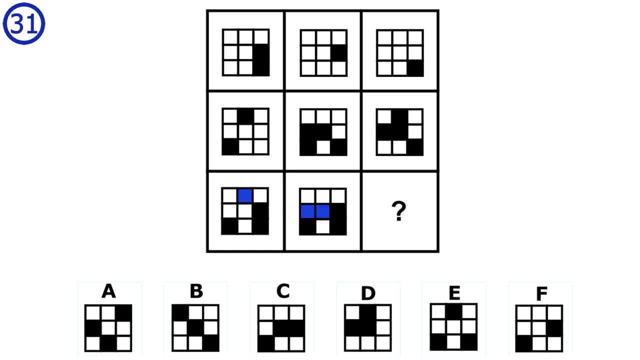 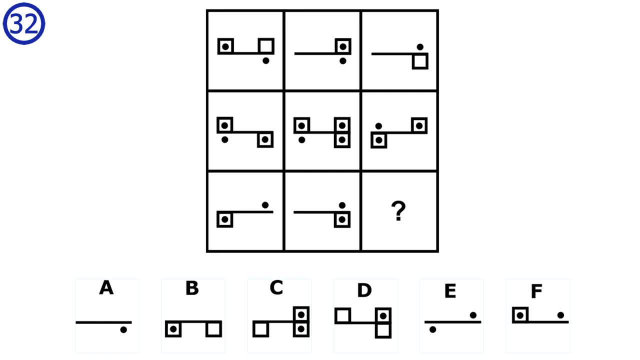 go by the third row. We have these three squares not in common. Adding them together produces answer D. Answer D is the correct solution, Puzzle 32.. If we look at the first row, the two first pictures have this square in the top right in common and this dot in the bottom right in common In the third picture, the. 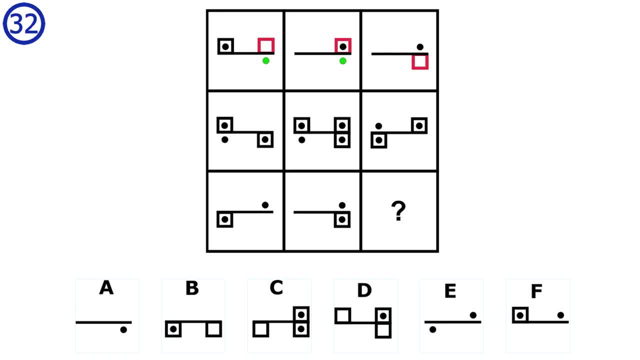 square in the top right is flipped over to the bottom right and the dot in the bottom right is flipped over to the top right. For the second row. we have this in common on the top half, which is flipped over to the bottom half in the third picture, and for the bottom. 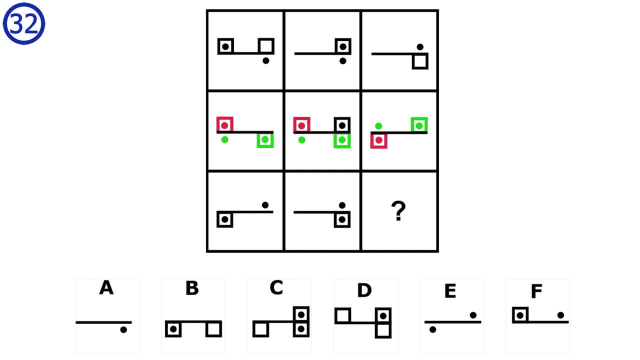 half. we have this in common, which again, is flipped over to the top side in the third picture. To solve the puzzle, we have to look at the third row and the only thing we have in common is this dot on the top right. After flipping the dot over to the bottom, we see: 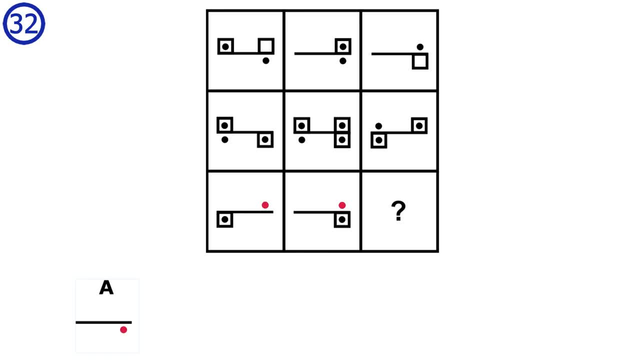 that the answer will only contain a dot on the bottom right. Answer A is the correct solution: Puzzle 33.. The first step to solving this puzzle is to see where there are similarities between the pictures. Personally, I see similarities on the top right to bottom left diagonals. 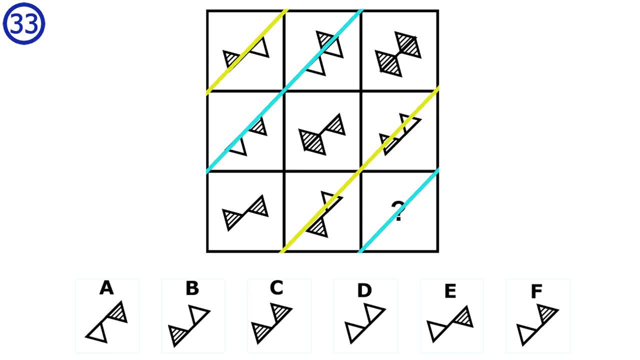 For example, in the purple diagonal, we see that the pictures are very similar. Now the way we move downwards in this diagonal is like this: Going from picture 1 to picture 2, we take the top right triangle and flip it to the bottom right so that it all lapses. 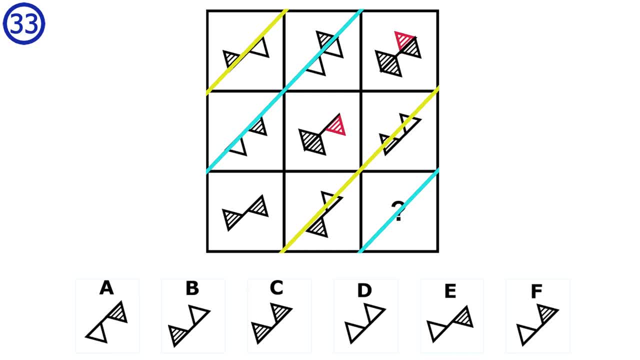 with the original triangle in that position. Going from picture 2 to picture 3, the bottom left triangle is flipped to the top left. Next, I want you to focus on the yellow diagonal. Going from picture 1 to picture 2. we flip the bottom right triangle to the top right. 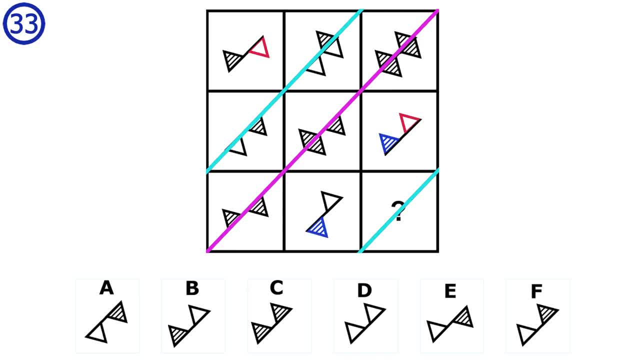 And going from picture 2 to picture 3, we flip the top left triangle to the bottom left. Notice that we flipped different triangles in this diagonal, meaning that when we go from picture 1 to picture 2, if we don't have the option to flip the bottom right triangle to the bottom left, And going from picture 2 to picture 3, we flip the top left triangle to the bottom left. Notice that we flipped different triangles in this diagonal, meaning that when we go from picture 1 to picture 2, if we don't have the option to flip the bottom left triangle to the bottom left, 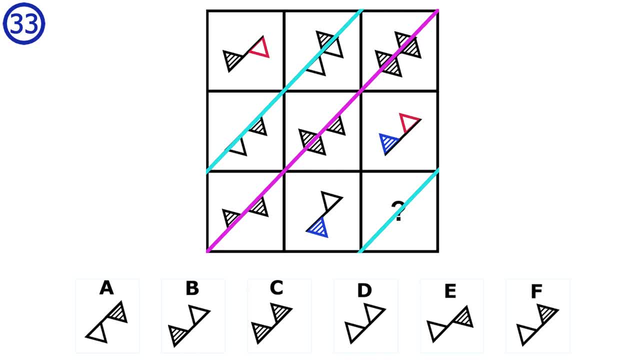 If we don't have the option to flip top right to bottom left, we flip bottom left to top right instead. And going from picture 2 to picture 3, if we don't have the option to flip bottom left to top left, we flip top left to bottom left instead. 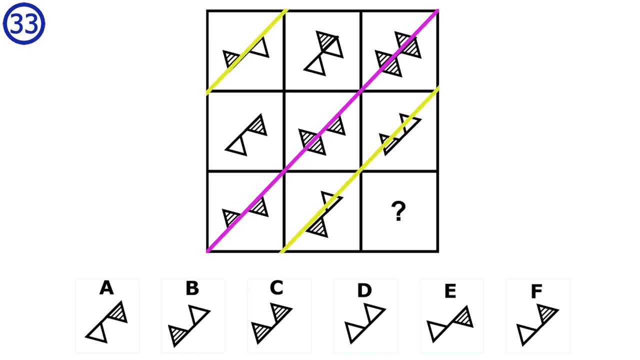 To solve the puzzle we have to focus on the light blue diagonal. Going from picture 1 to picture 2, we flip the top right triangle to the bottom right. And going from picture 2 to the answer, we flip bottom left to the top left. Only answer D and E has this white. 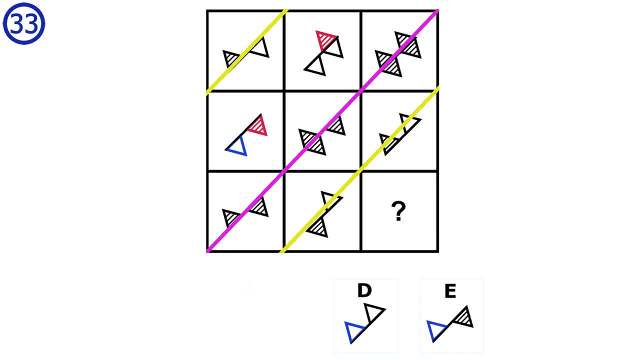 triangle on the top left, so we can eliminate all the other answers. The answer should also have this striped triangle in the bottom right, since it wouldn't change in any way from picture 2 to picture 3.. This leaves answer E as the correct solution. 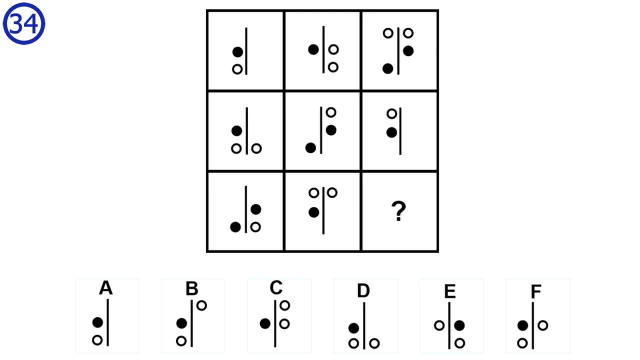 Puzzle number 34.. This is another puzzle where I see a pattern in the top right to bottom left diagonals. First of all, we can see that the pattern of the black dots repeat on these diagonals For the pattern of the white dots. I will go over each of the diagonals, Starting 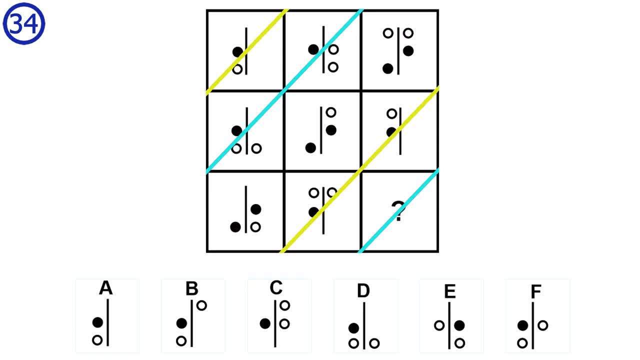 off with the purple diagonal. we have two white dots in the first picture. I'll mark them in the red and blue. Going from picture 1 to picture 2, the dots move in the red and blue. The dots move in one position in clockwise direction. The blue dot moves to the top right corner, while the 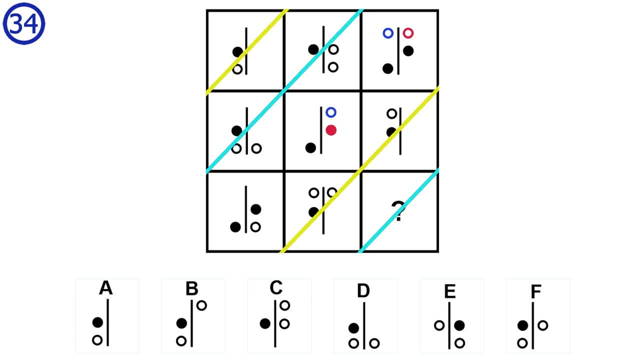 red dot moves under the black dot on the middle right. Going from picture 2 to picture 3, the red dot moves to the bottom right corner, while the blue dot moves under the black dot in the middle right. Next going through the yellow diagonal In the first picture, the red dot is hiding under. 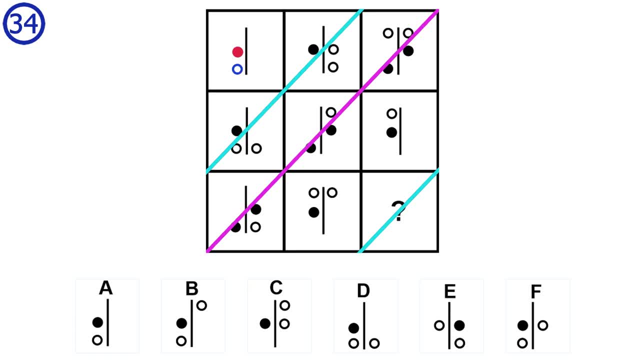 the black dot while the blue dot is out in the open. Going from picture 1 to picture 2, we move the dots once in clockwise direction, which leads to the red dot being in top left and the blue dot under the black dot in the middle. 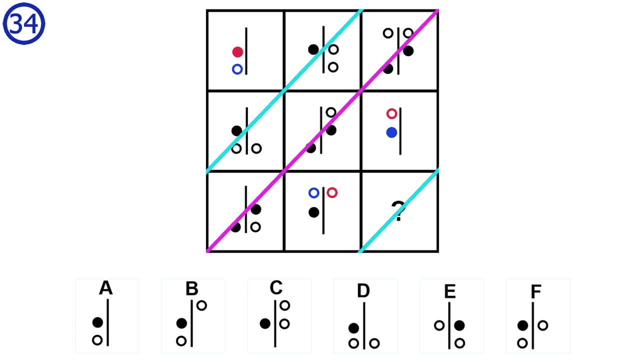 left. Going from picture 2 to picture 3, we move the dots once in clockwise direction. The red dot ends up in the top right, while the blue dot ends up in the top left. To solve the puzzle, we go by the light blue diagonal, where the answer is in. 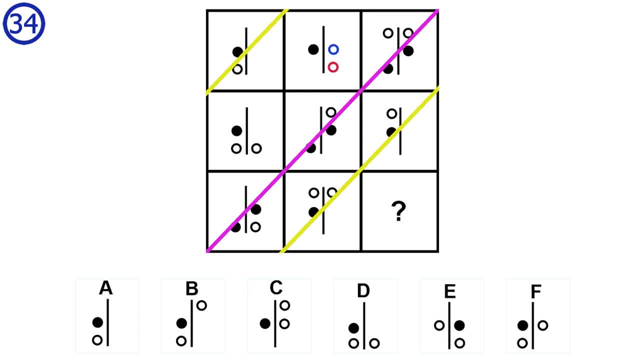 In the first picture the two dots can be seen on the bottom right and the middle right. In the second picture they are moved once in clockwise position, leading to the red dot being on the bottom left and the blue dot being on the bottom right. Going from picture 2 to the answer, we see that the red dot moves under the black dot. 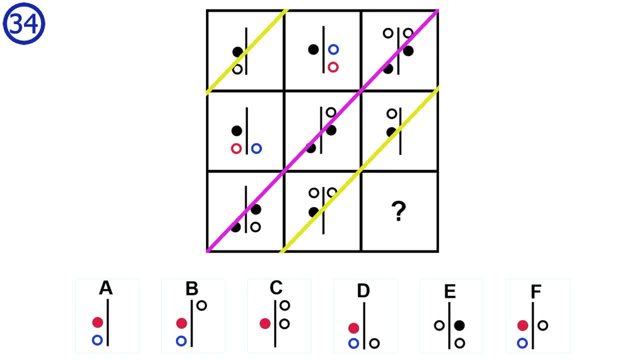 in the middle left and the blue dot moves to the bottom left. Answers C and D does not have a dot in the bottom left, so we can eliminate the answers. If we look at answer B, D and F, they each have an extra dot which is not explained by. 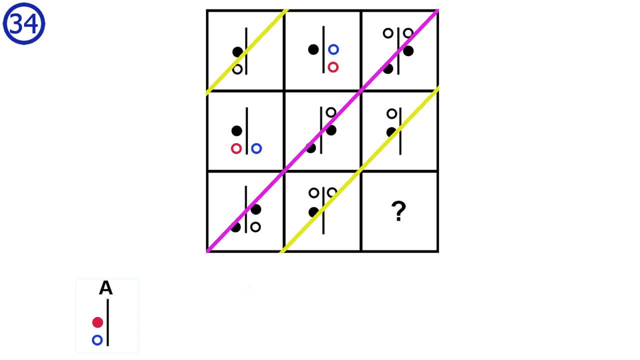 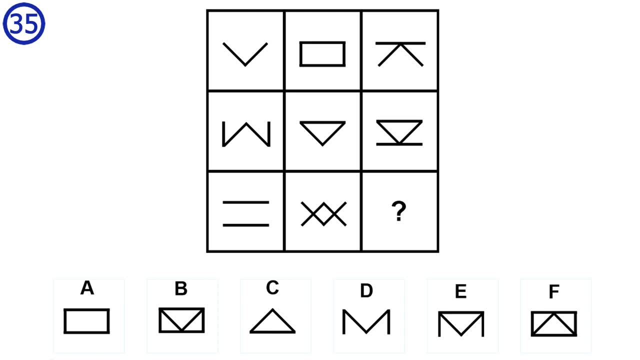 the pattern in the diagonals. so we can eliminate these answers. Answer A is the correct solution. Puzzle number 35. The final puzzle of the IQ test. The way I solved the puzzle was by looking at the repetition in the diagonals. Looking at the top left to bottom right diagonal, we see repetition of shapes.